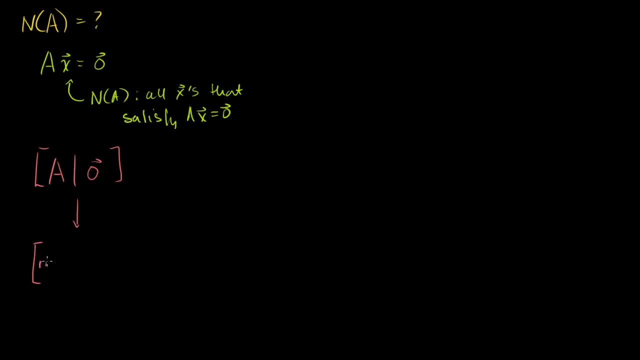 The left-hand side would go into reduced row echelon form. Let's call that reduced row echelon form of A, And then the right-hand side is just going to stay 0, because you performed the same row operations. But when you perform those row operations on 0, you just get. 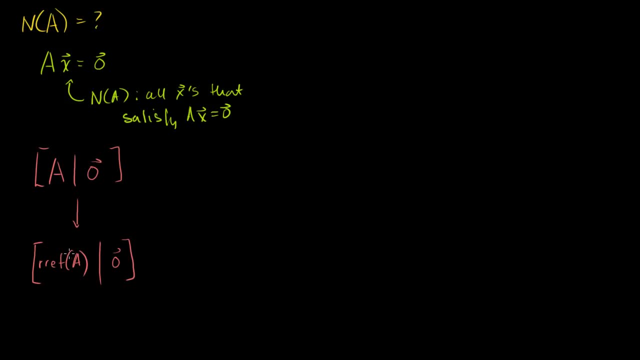 the 0 vector right here, And then, when you create the system back from this- right here, because these two systems are equivalent- you're essentially going to have your solution set. look something like this: You're going to have your. let me write it like this: 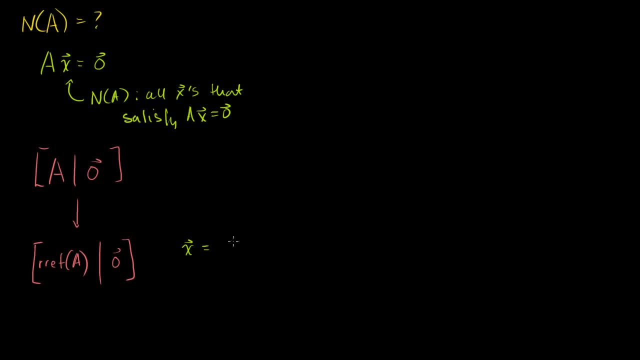 Your solution set is going to be equal to some scalar multiple. you know, Let's say that Of your free variables, Your free variables are going to be the scalar multiples, And you've seen this multiple times. So I'll say it's fairly general. 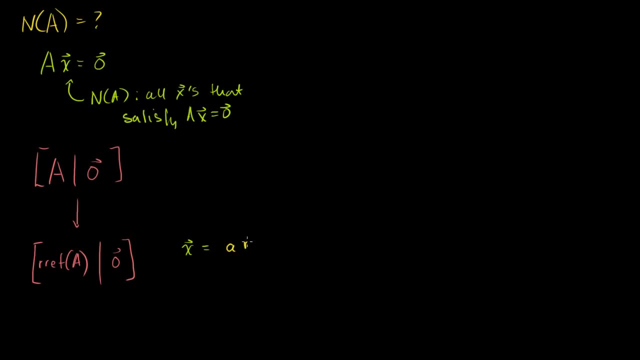 But it's going to be some multiple times. let's say vector 1 plus some other scalar times vector 2. These scalars tend to be your free variables Times vector 2 all the way to I don't know whatever c. 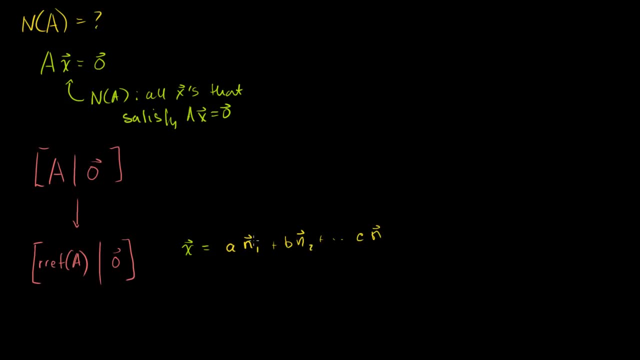 times your nth vector. I'm just trying to say general. We haven't seen any examples that had more than two or three vectors here, But this is what essentially: your null space is spanned by these vectors. right there You get an equation, you get a solution set that looks: 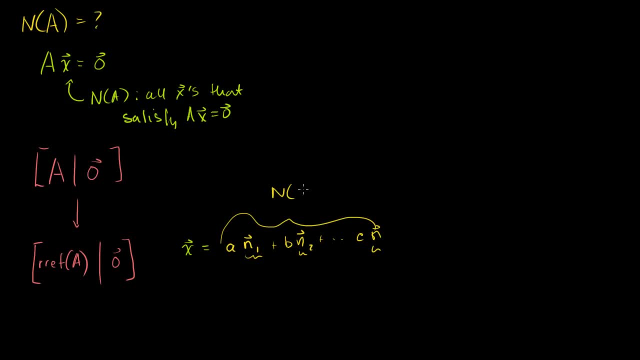 something like that And you call that your null space. We've done that multiple times. Your null space is that. So it's all the linear combinations or it's the span of these little vectors that you get here: n1,, n2, all the way to nn. 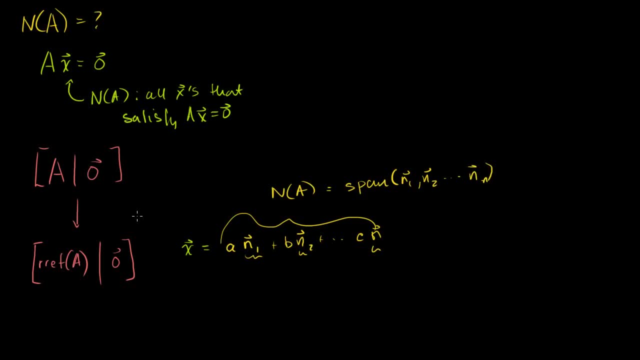 This is nothing new. I'm just restating something that we've seen multiple, multiple times. We've actually did this in the previous video. I just maybe never wrote it exactly like this. But what about the case when you're solving the inhomogeneous equation? 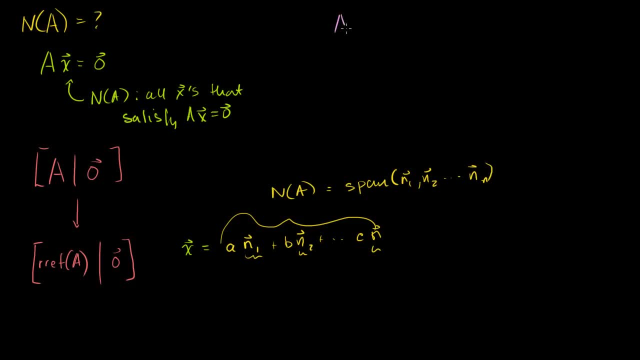 So the inhomogeneous equation looks like this. So if I want to solve, Ax is equal to b. I would do something very similar to this. I will create an augmented matrix. I have a on the left-hand side and I'd put b on the. 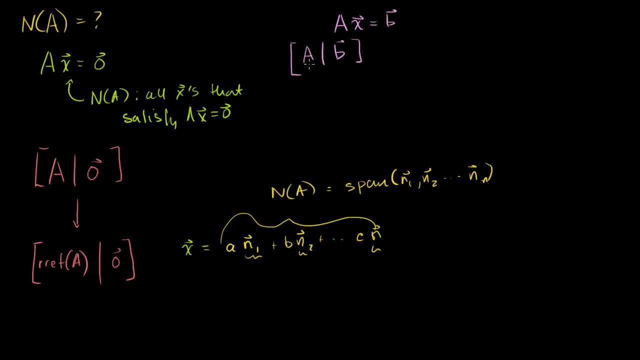 right-hand side And then I'll perform a bunch of row operations to put a into reduced row echelon. So I'll put a into reduced row echelon, So let me do that. So this left-hand side will be the reduced row echelon form of A. 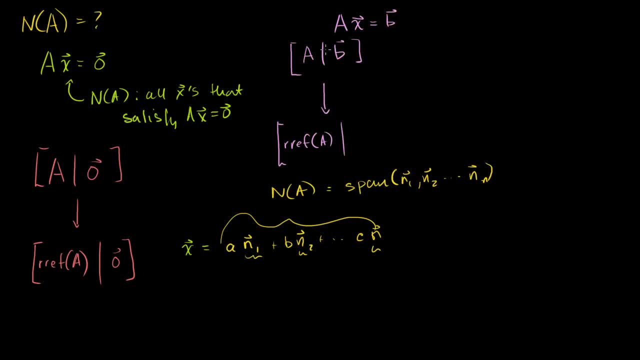 And then the right-hand side. whatever operations I did on A, I have to do on the entire row, So I'll also be doing them to b, So I'll have some new vector here. Maybe I'll call it the vector b prime. 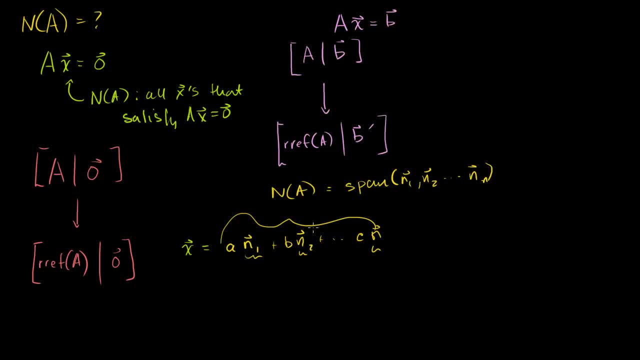 It's going to be different than b, but let's just call it b prime. And so when you go back to your, I guess, when you go out of the augmented matrix world and rewrite it as a system and you solve for it, 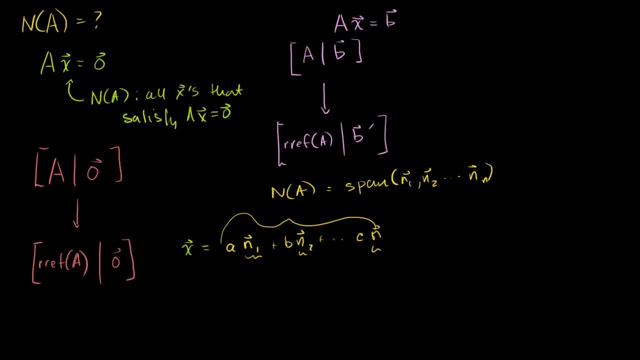 and we did this in the last video- you'll get your solution set, Your solution set that satisfies. this is going to be: x is going to be equal to this b prime. whatever this new vector is this b prime plus something that looks exactly. 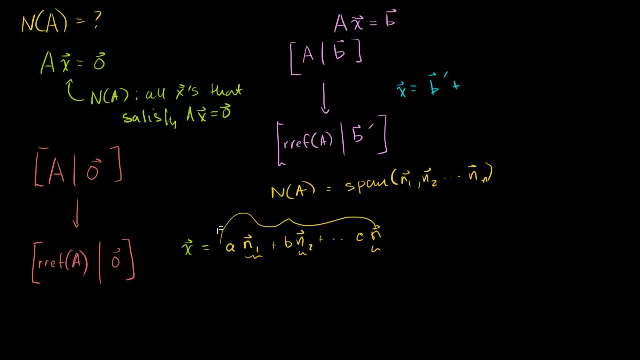 like this. That looks exactly like that, In fact, I'll copy and paste it. It'll look exactly like this. Let me see if it did copy. Let me copy and paste it. Edit copy and then let me paste it. 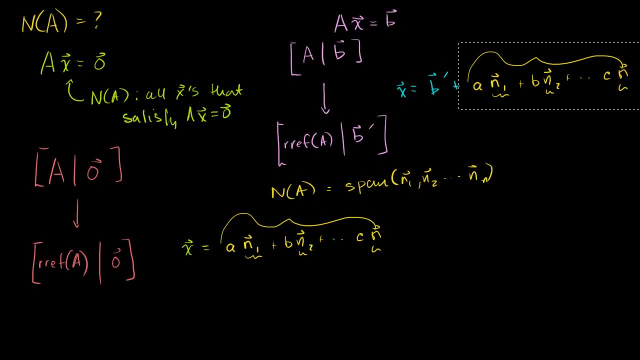 So it'll look something that looks exactly like that And we said in the last video that that you can kind of, given this, you can kind of think of: the solution set to the inhomogeneous equation is equivalent to some particular solution is equal to some particular solution. let's call. 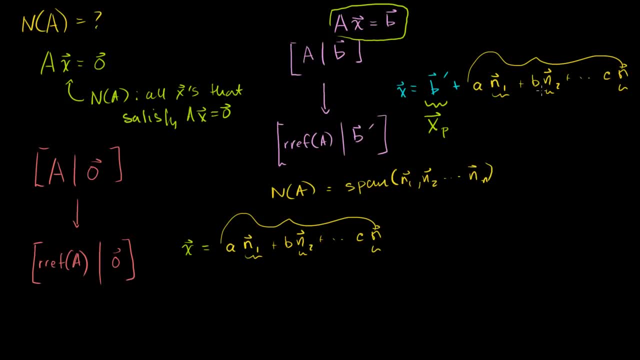 that x, Some particular solution plus some member of your null space. So you could say it's plus some homogeneous solution. So if you just pick particular values for a, b and c, all of the different multiples of the vectors that span your null. 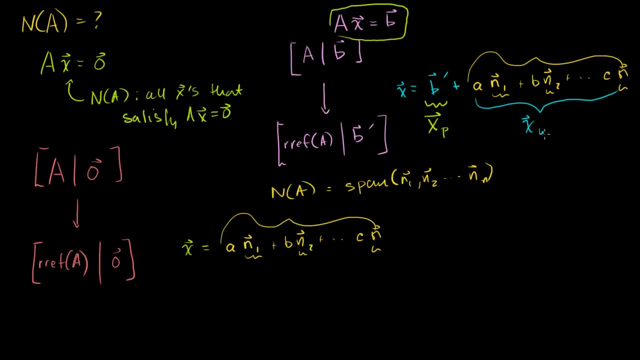 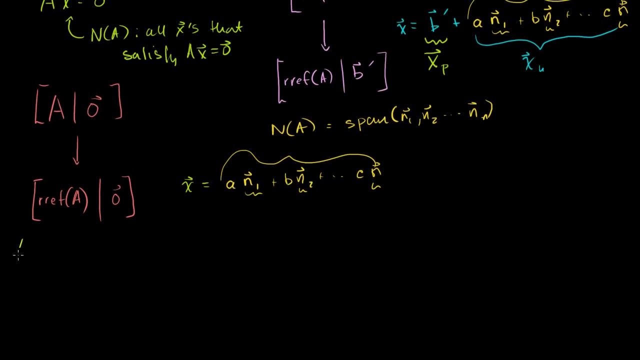 space, you'll get some particular homogeneous solution. So what I implied in the last video- and I didn't show it to you rigorously- is that any solution to the inhomogeneous system. let me write it this way: Any solution, and do it in white. 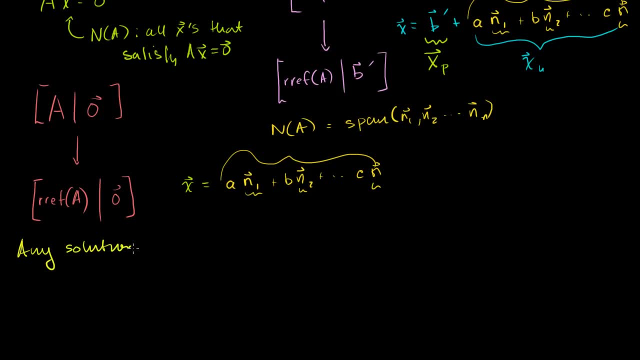 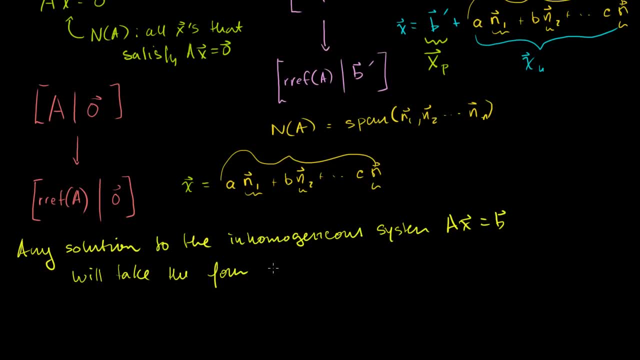 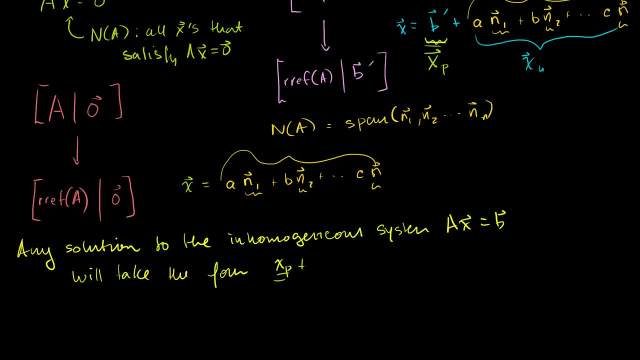 b prime vector Plus some homogeneous solution. So some member of the null space. Now I didn't prove it to you, but I implied that this is the case, And what I want to do in this video is actually do a little bit of a more rigorous proof. 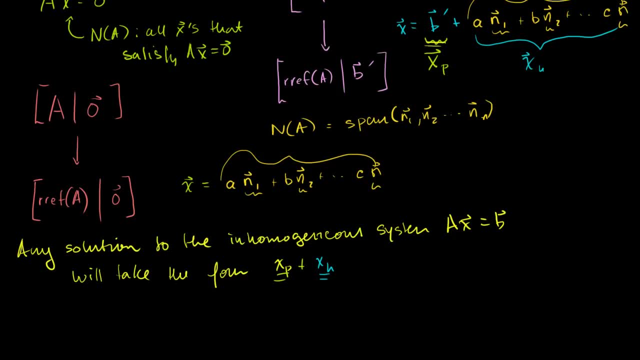 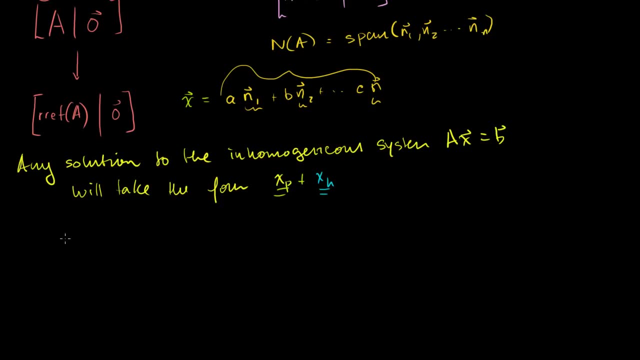 But it's actually fairly straightforward. So let's first of all verify that this is a solution. So let's just put this into our original equation. So remember our original equation was: Ax is equal to b. So let's verify: So is. let me write it as a question: is that particular? 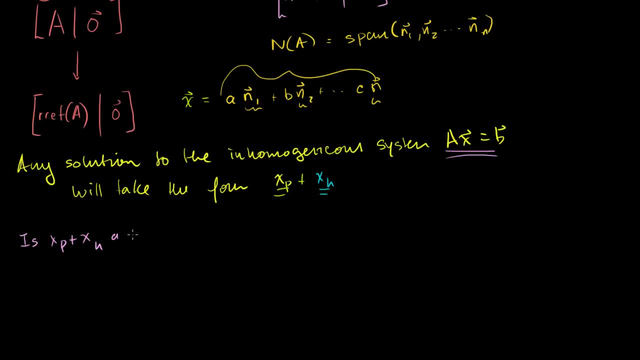 solution plus some homogeneous solution. a solution To Ax is equal to b. Well, to do that, you just put that in the place of x. So let's try it out. So a times this guy right here times some particular solution plus some homogeneous solution is going. 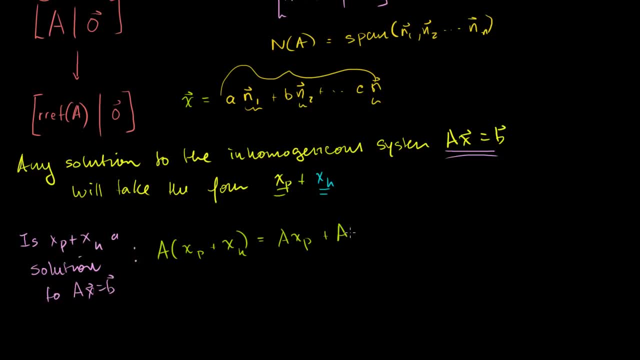 to be equal to a times the particular solution plus a times some member of my null space. And what is this equal to? That is going to be equal to b? Right, We're saying that this is a particular solution to this equation. 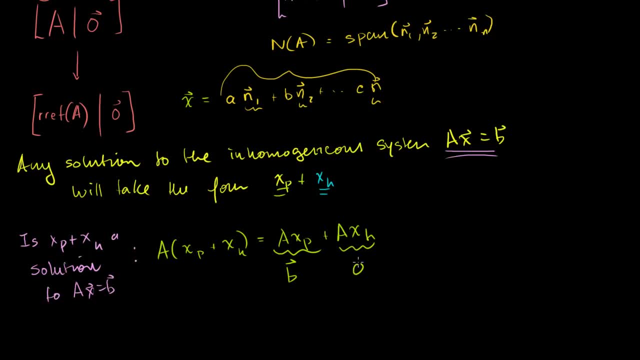 That is going to be equal to b And that this is going to be equal to the 0 vector, Because this is a solution to our homogeneous equation. So this is going to be equal to b plus 0, or it's equal to b. 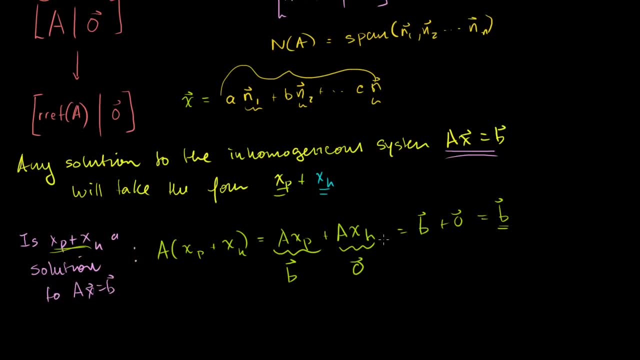 So a times this vector right here is indeed equal to b. So this is a solution. This is a solution, yes. Now the next question is: does every solution to the inhomogeneous system, Or does any solution to the inhomogeneous system take this? 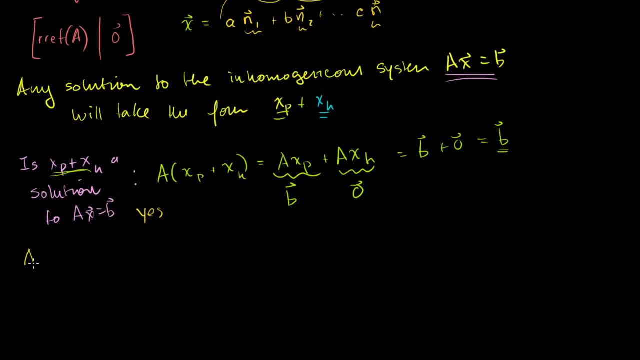 form. So does any solution x to ax equal to b. take the form x is equal to some particular solution plus a member of our null space or plus a homogeneous solution. So to do that, Let's take, Let's test out what happens when we multiply the vector a. 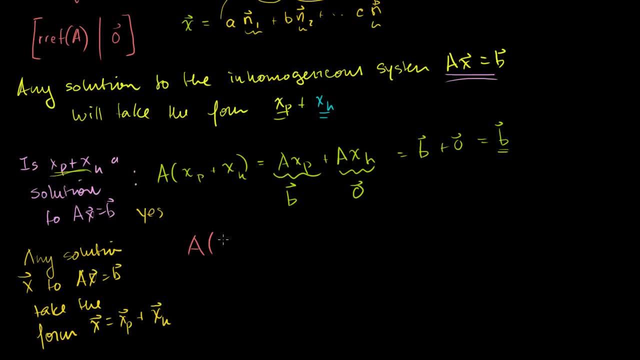 times x. Let me write it this way: Let's say that x is any solution to ax is equal to b. Let's start off with that And let's see what happens when we take a times x minus some particular solution, Some particular solution to this. 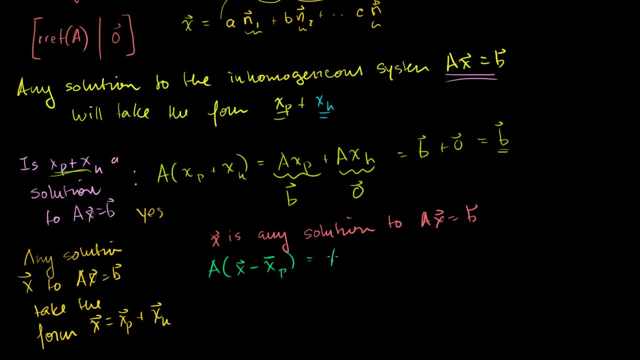 So when we distribute the matrix vector product, you get a times our any solution, minus a times our particular solution. Now, what is this going to be equal to? We're saying that this is a solution to ax equal to b. So this is going to be equal to b. 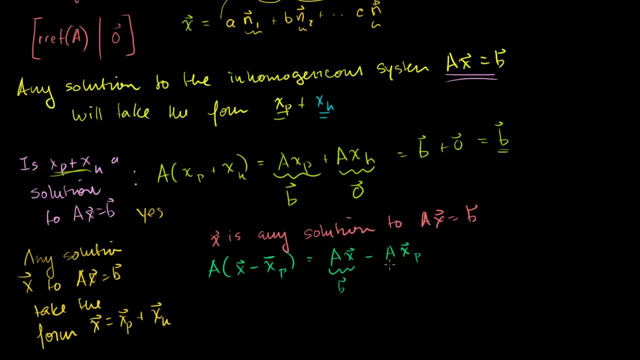 And, of course, any particular solution to this. when you multiply it by a is also going to be equal to b, So it's going to be b minus b. So that's going to be equal to the 0 vector. So that's going to be b minus b. So that's going to be equal to the 0 vector. 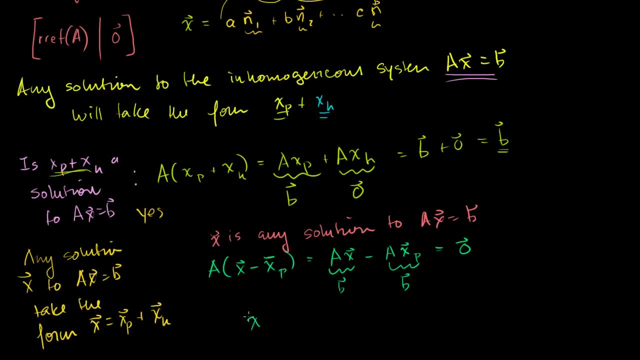 Or another way to think about it is the vector x minus. our particular solution is a solution to a times x is equal to 0. Think about this: If you take this in parentheses right here and you put it right there, when you multiply it times a, you get the 0. 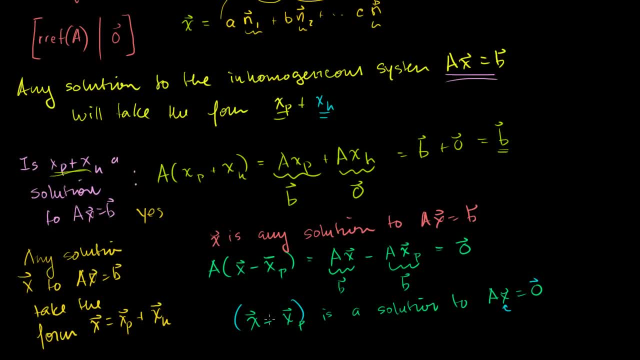 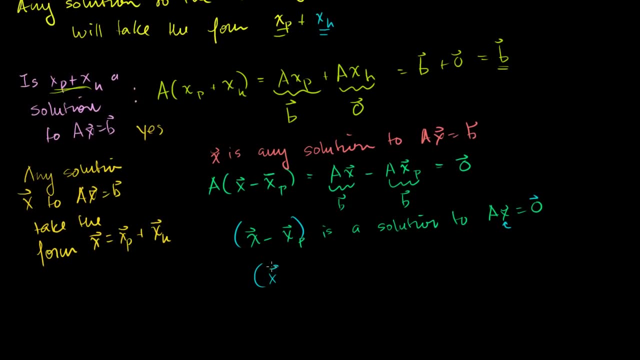 vector. We just did that. You get the 0 vector, because when you multiply each of these guys by a, you get b, And then you get b minus b, And so you get 0. So you can say that x minus, so any solution, x minus the. 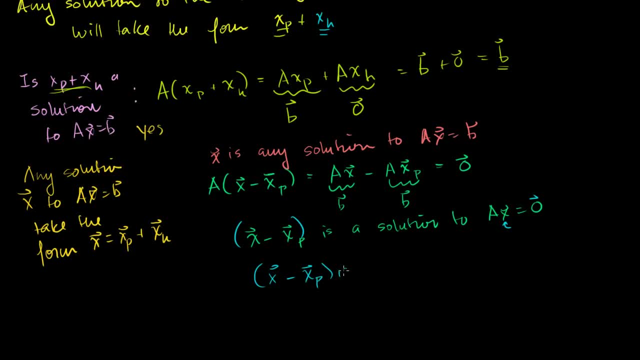 particular solution of x is a member of our null space. By definition, your null space is all of the x's that satisfy this equation, And let's say so. since it's a member of our null space, we can say that it is equal to, so our any solution minus our. 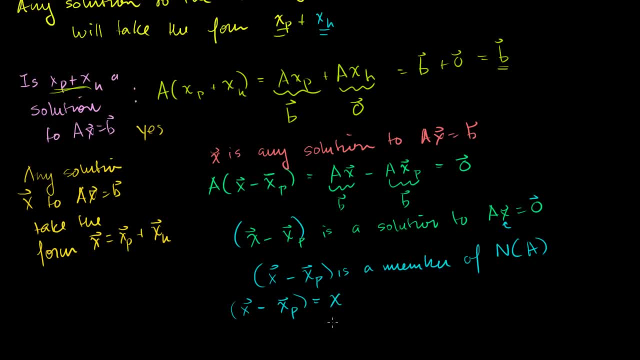 particular solution is equal to some member of our null space. We could say that it's equal to a homogeneous solution. There might be more than one A homogeneous solution Now, if we just add our particular solution to both sides of this. 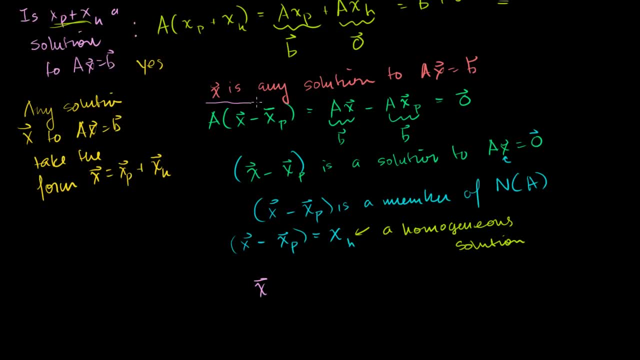 We get that any solution- Remember we assume that x is any solution to this- That any solution is equal to our homogeneous solution- is equal to a homogeneous solution plus our particular solution. So we've proven it both ways: That this is a solution to our inhomogeneous equation and 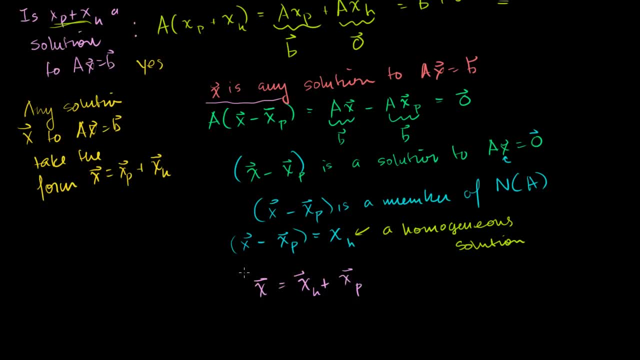 that any solution to our inhomogeneous equation takes this form, right here. Now, why am I so confused? Why am I so confused? Why am I so concerned with this? You know, I've been kind of fixated on this inhomogeneous 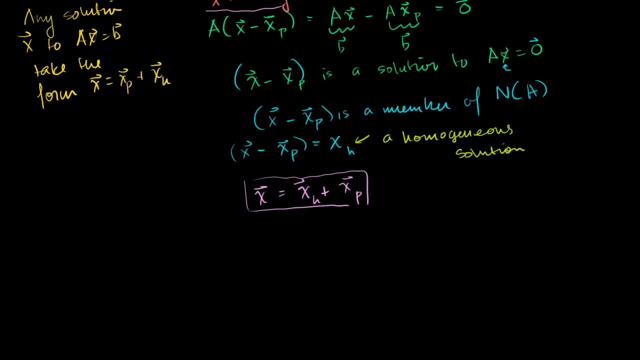 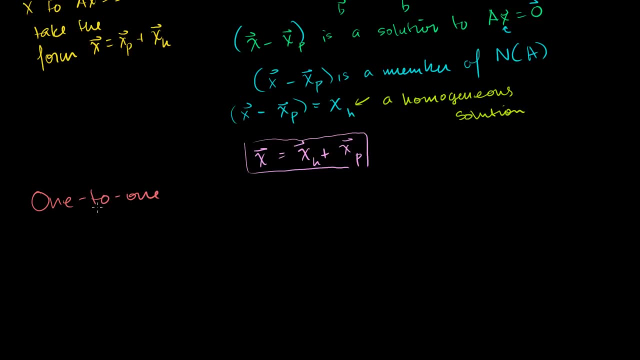 equation for some time, But we've been talking about the notion of a transformation being 1 to 1.. A transformation being 1 to 1. That was one of the two conditions for a transformation to be invertible, Now to be 1 to 1, so let me draw a transformation here. 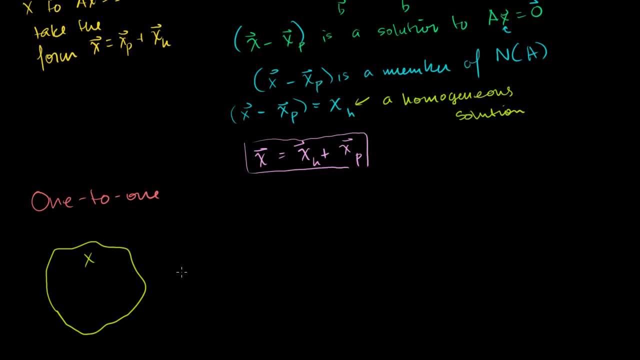 So let's say this is my domain x, and this is my co-domain right here, y, And I have a transformation that maps from x to y In order for t to be 1 to 1, so I'll write it like this: 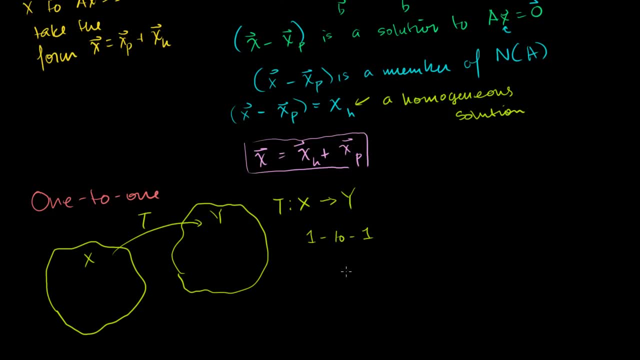 1 to 1.. In order for t to be 1 to 1, that means for any b that you pick here, for any b that is a member of our co-domain, there is at most 1 solution to a times x. 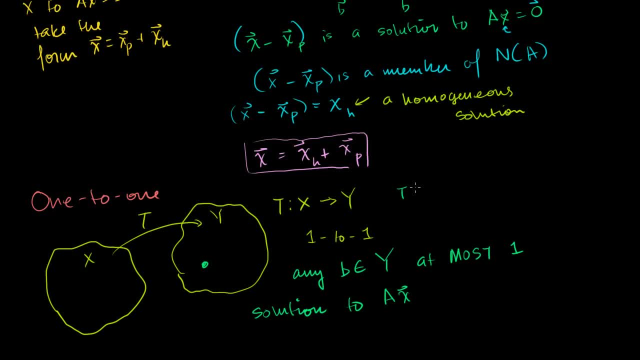 And I'm assuming that a is our transformation matrix, so we can write our transformation t as being equal to some matrix times our vector in our domain. So this would be ax if this is x right here. So t would map from that to that, right there. 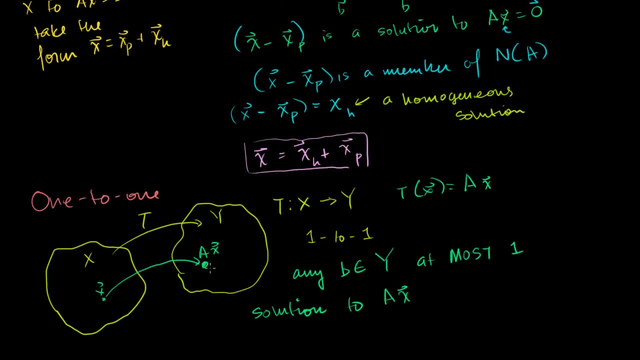 So in order for our transformation to be 1 to 1, that means you pick any b here- there has to be at most one solution to. ax is equal to b, Or another way to say that is that there is at most one guy. 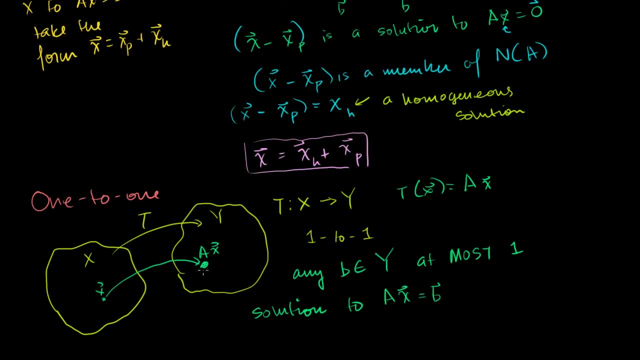 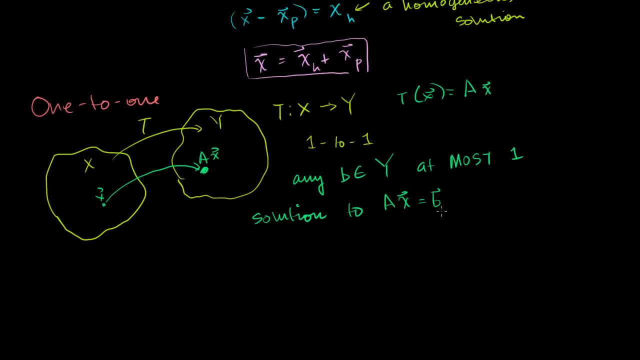 that maps into that element of our co-domain. There might be none, So there could be no solutions to this, but there has to be at most one solution. Now, we just said that any solution to an inhomogeneous, So we just said that any. let me write it in blue: 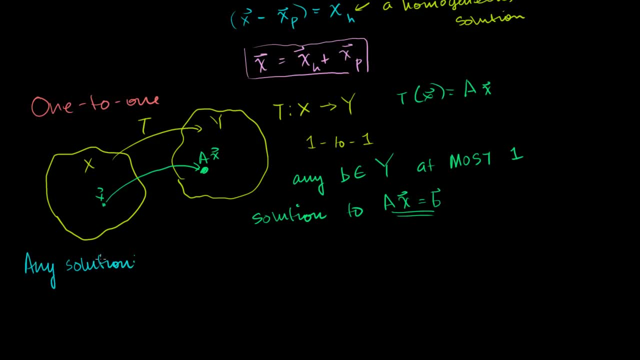 Any solution takes the form if there is a solution. So if there isn't a solution, that's fine, That'll still satisfy 1 to 1.. But if there is a solution, any solution is going to take the form x particular plus a member of your null space. 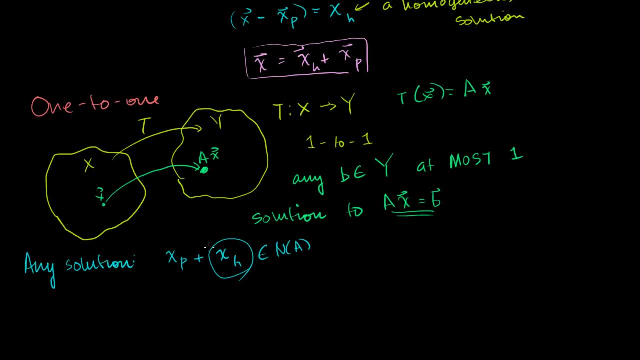 Where this guy right here is a member of the null space. This thing right here just applies to that guy right here. Any solution, if they exist. If there are no solutions, that's fine, You can still be 1 to 1.. 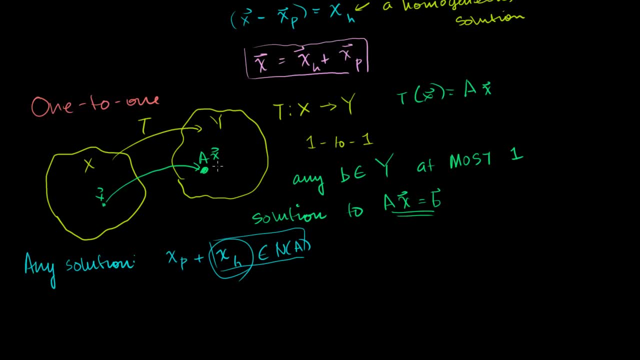 But if you do have a solution, you can have at most one person that maps to it, And any solution will take this form. I just showed you that Now, in order to be 1 to 1, this can only be one solution. 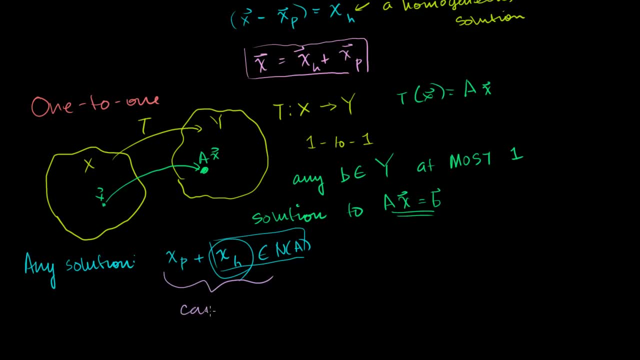 The solution set can only be one solution. This can only be one solution. We can only have one solution here, right? What does that mean? That means that this guy right here cannot be more than one vector. It just has to be one vector. 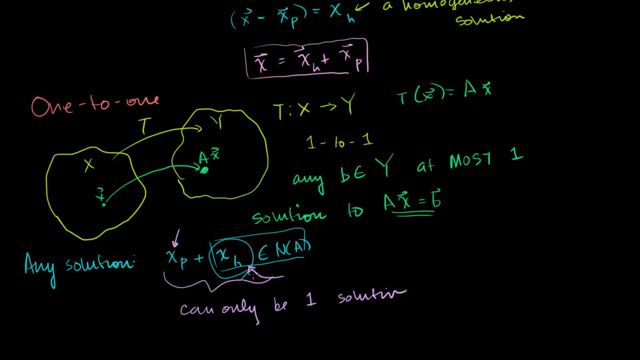 This is only. There's only one particular solution right there, But this guy right here has to be well, for any solution set, depending on how you define it, there's only one particular vector there, But this guy, the only way that you're only going to have one. 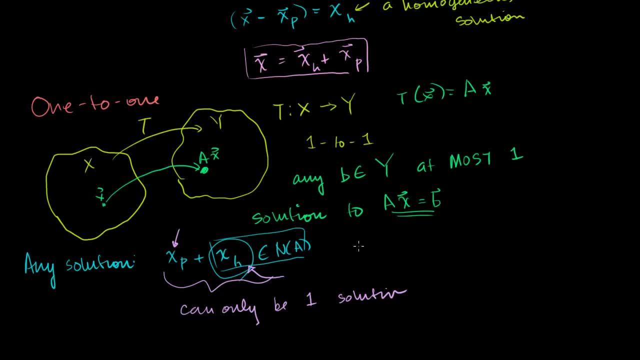 solution is: if your null space is trivial, if it only contains the 0 vector, Your null space will always, at minimum, contain the 0 vector. In the last video, I think I just off the cuff, said: oh, your null space has to be empty. 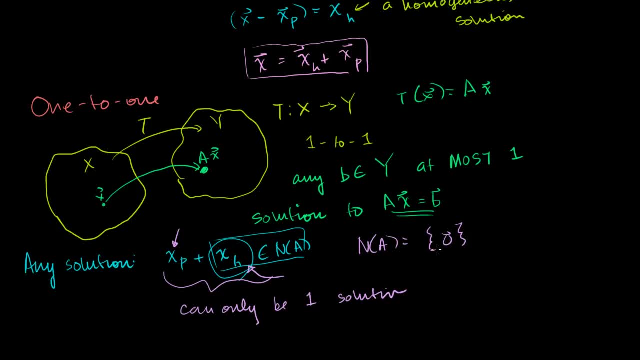 But no, Your null space will always contain the 0 vector. Your null space will always, at minimum, contain the 0 vector. Your null space will also will always, by definition, by the fact that it is a subspace, it will always contain a 0 vector. 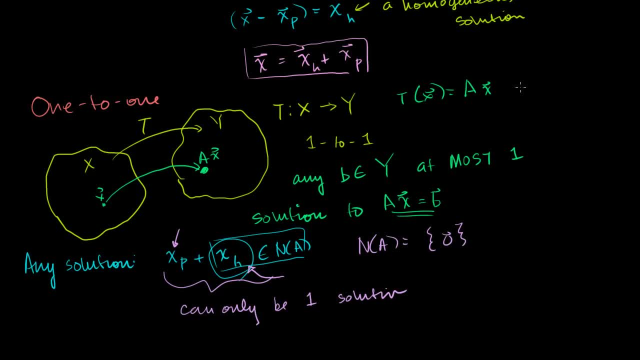 You can always multiply a times 0 to get 0. So your null space will always contain that. But in order to have only one solution, your null space can only have the 0 vector, so that this can only be 0, and 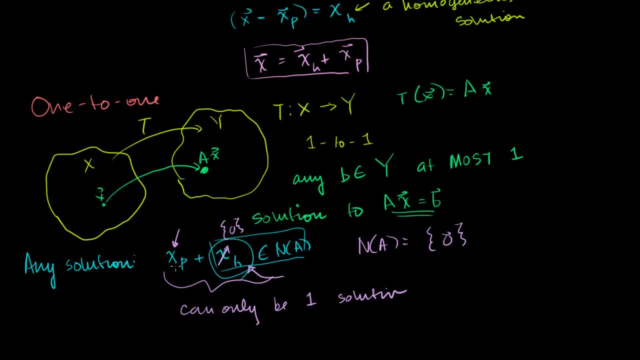 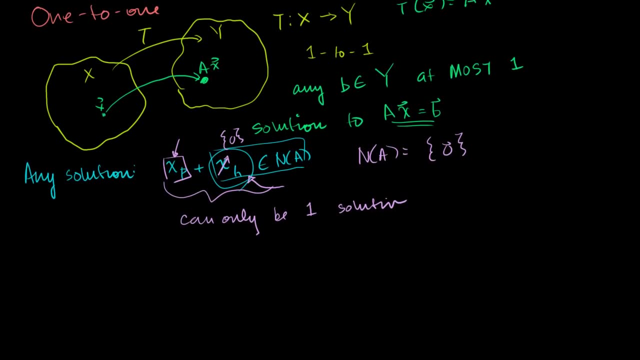 so that your only solution is going to be the particular solution that you found, depending on how you got there, But it's only going to be your particular solution. So let me put this this way: So, 1 to 1, in order to be 1 to 1,, your null space of your 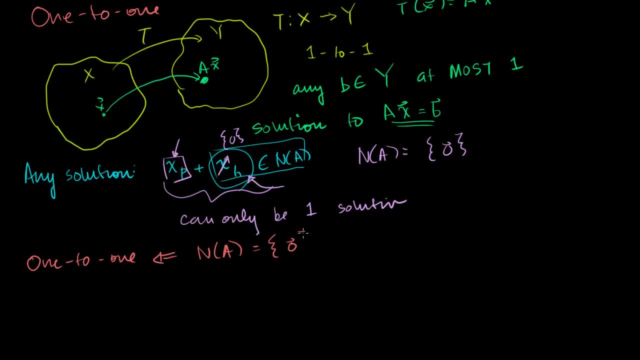 transformation matrix has to be trivial. It has to contain only the 0 vector. Now, we've covered this many, many videos ago. What does it mean if your null space only contains the trivial vector? Let me make this clear. So if your transformation vector looks like this: a1,. 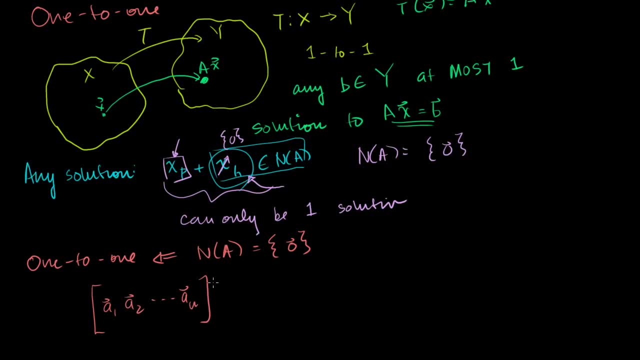 a2, all the way to an, and you're multiplying it times x1,, x2, all the way to xn, and the null space is all of the x's that satisfy this equation 0, and you're going to have m0's right there. 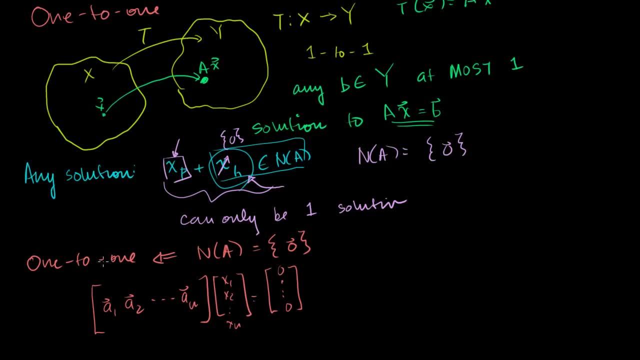 So if your null space is trivial- and we're saying that that is a condition for you to be 1 to 1, for your transformation to be 1 to 1, the transformation that's specified by this matrix. If your null space is trivial, what does that mean? 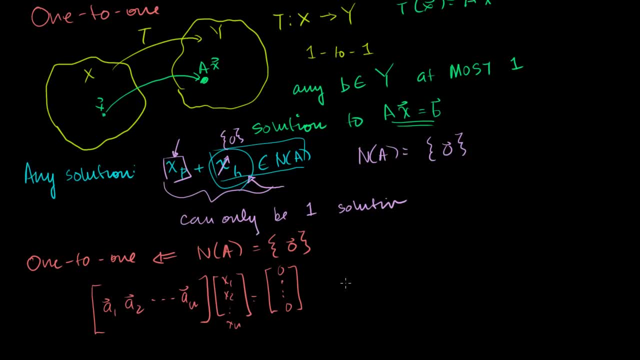 That means that the only solution to another way of writing this is: x1 times a1 plus x2 times a2, all the way to xn times an is equal to the 0 vector. These are equivalent statements right here. I just multiplied each of these terms times these respective. 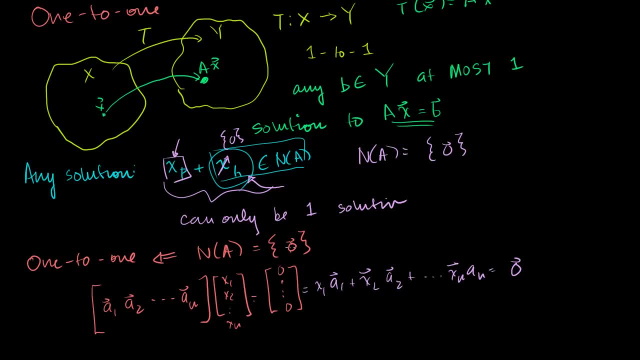 column vectors. These are the same thing. Now, if you say that your null space has to be equal to 0, you're saying that the only solution to this equation is right here, the only scalars that satisfy this equation. Sorry, these aren't me actually, because I wrote the 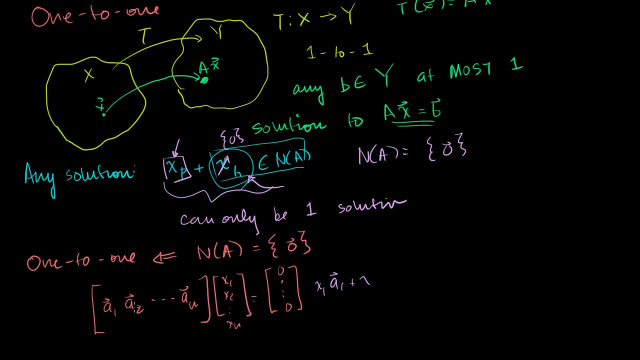 scalars as vectors. So this guy right here, this statement right here, is equivalent to x1 times a1 plus x2 times a2 plus all the way to xn times an, is equal to the 0 vector where the x1's through xn's are scalars. 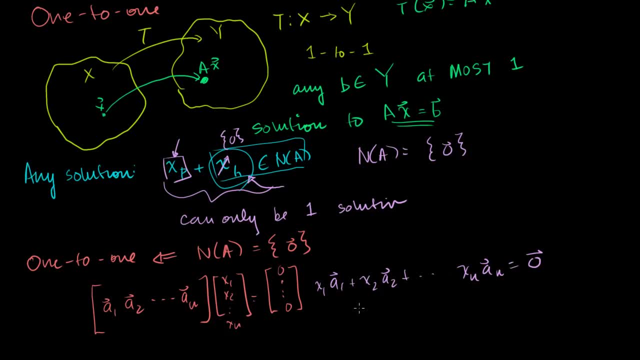 Now if we say the null space is 0, we're saying the only way this is satisfied is if your x1, all the way to xn, is equal to 0. And this means this is our definition actually of linear independence. 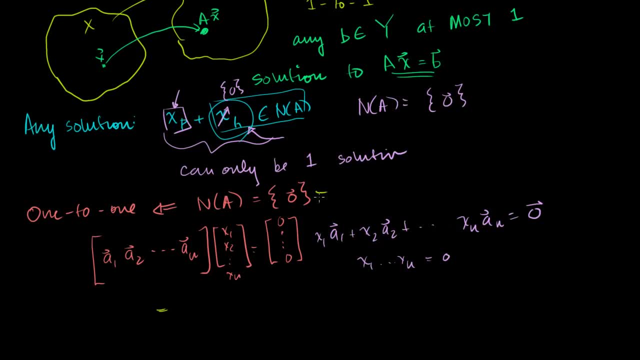 That means that a1, so the null space being 0, also means that your column vectors of a, your column vectors. let me write it this way: it also means that a1,, a2, all the way through an linearly independent. 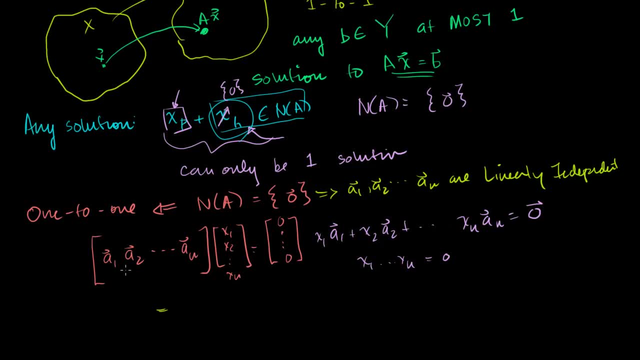 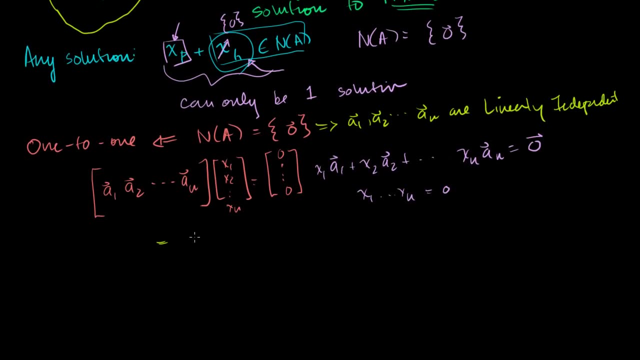 Now, what does that mean? If all of these guys are linearly independent, what is going to be the basis for your column space? Remember, the column space is the span. The column space of a is equal to the span of a1,, a2, all the. 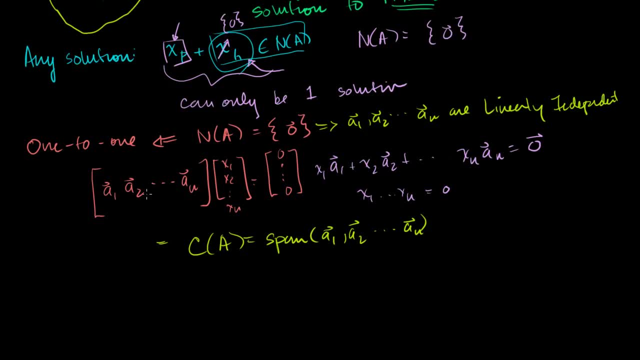 way to an. Well, we just said, if we're dealing with a one-to-one or, or one of the conditions, or the condition to be 1 to 1, is that your null space has to be 0, or only. 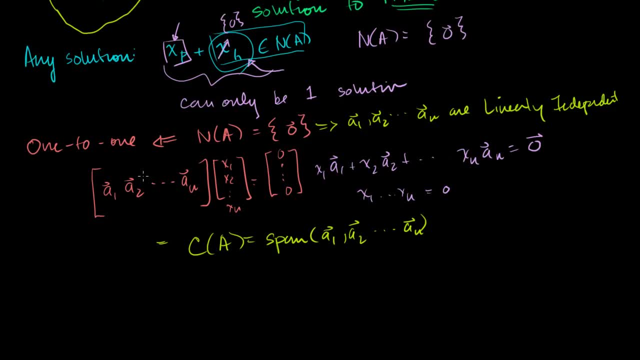 contains a 0 vector. If your null space contains a 0 vector, then all of your columns are linearly independent. If all of these columns span your column space and they're linearly independent, then they form a basis. So that means that a1,, a2,, all the way to an, are a basis for. 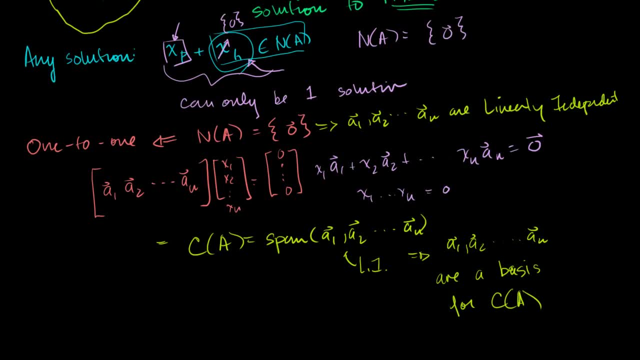 our column space. And then that means, if all of our column vectors here are linearly independent, they obviously span our column space by definition, and they all are linearly independent. they form the basis, So the dimension of our basis, So the dimension. 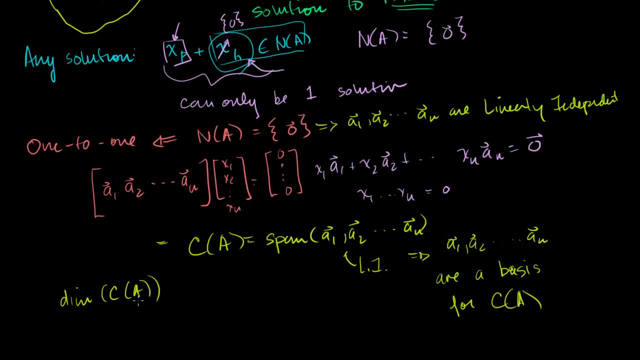 Of our column space, The dimension of our column space, That's essentially the number of vectors you need to form the basis. It's going to be equal to n. We have n columns, So it's going to be equal to n. Or another way to say it is that the rank of your matrix. 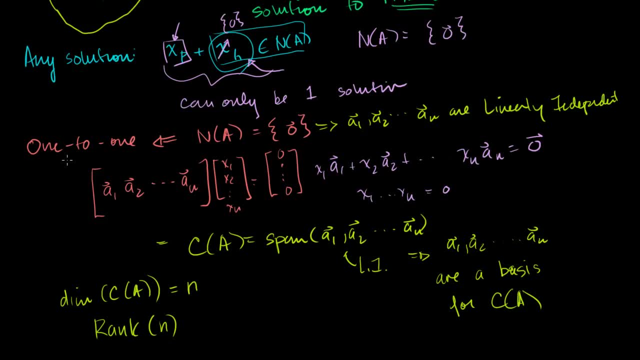 is going to be equal to n. So now we have a condition for something to be 1 to 1.. Something is going to be 1 to 1 if, and only if, the rank of your matrix is equal to n, And you could go both ways. 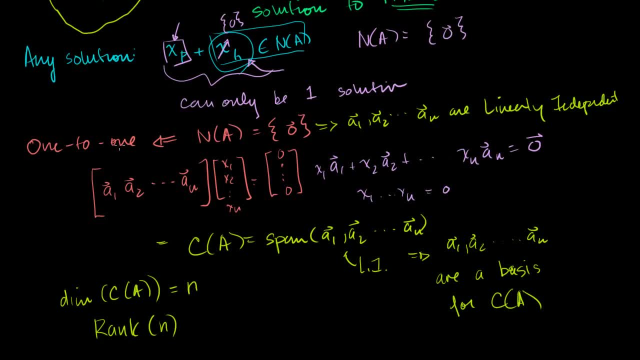 If you assume, If you assume something Is 1 to 1, then that means that it's null space here has to only have the 0 vector, So it only has one solution. If it's null space only has the 0 vector, then that means it's. 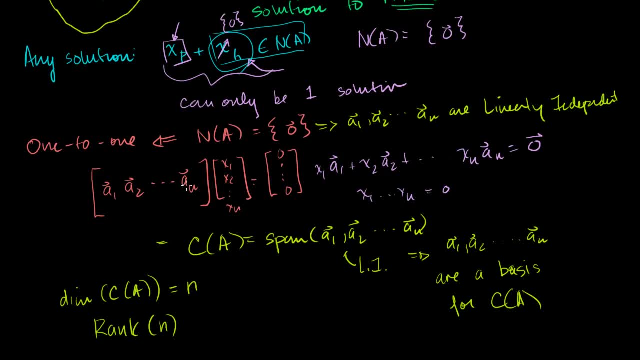 columns are linearly independent, which means that they all are part of the basis, Which means that you have n basis vectors or you have a rank of n. Go the other way. If you have a rank of n, that means that all of these guys. 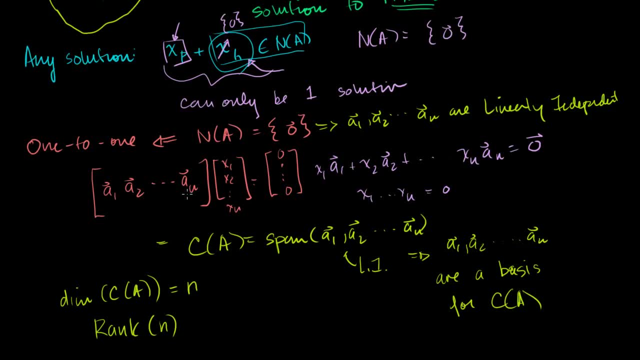 are linearly independent. If all of these guys are linearly independent, then the null space is just the 0 vector, And then that The null space is just the 0 vector, This part of your solution disappears, And then you're only left with one solution. 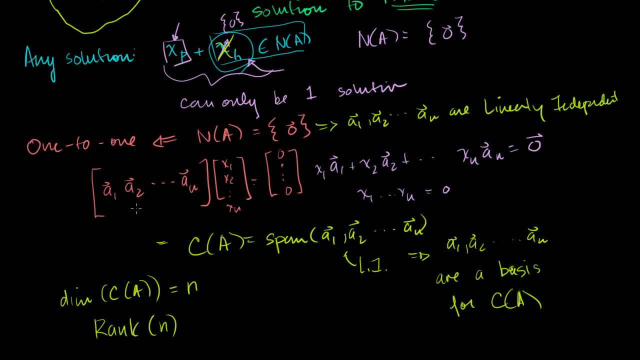 So you're 1 to 1.. So you're 1 to 1 if, and only if, the rank of your transformation matrix is equal to n. 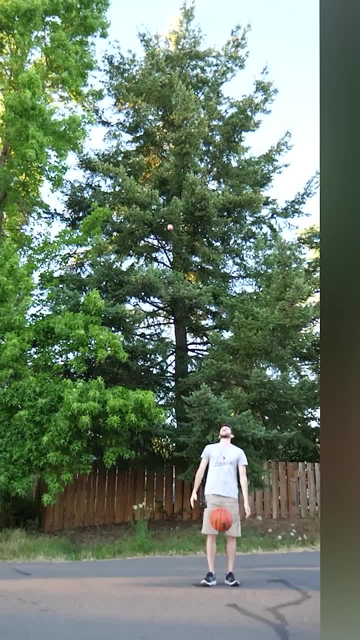 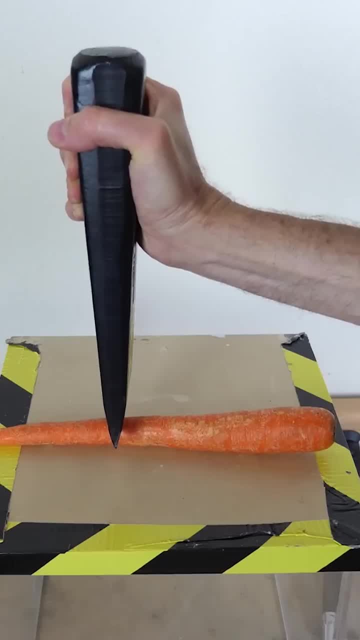 Momentum equals mass times velocity. so when you transfer the momentum from a heavy thing to a lighter thing, then that makes the lighter thing have a much higher velocity, which you can easily see in the stacked ball demonstration. The opposite is also true. This sharp wedge. 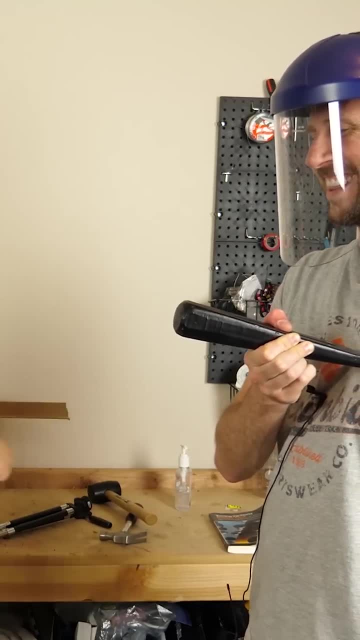 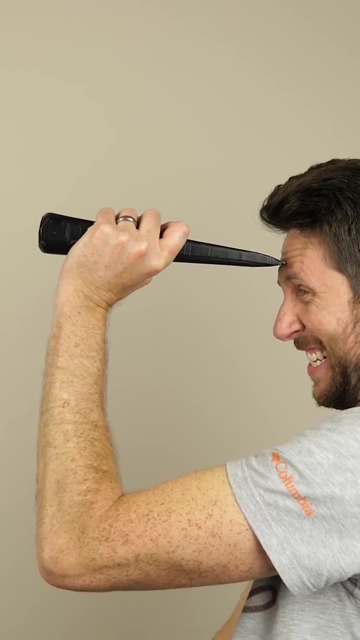 has a large mass. so that means that when my wife hits it with this low mass stick, the wedge doesn't get much forward velocity, so it can't pierce me. Now let's get a little more daring here, So you can see that when you have something with a smaller mass hitting, 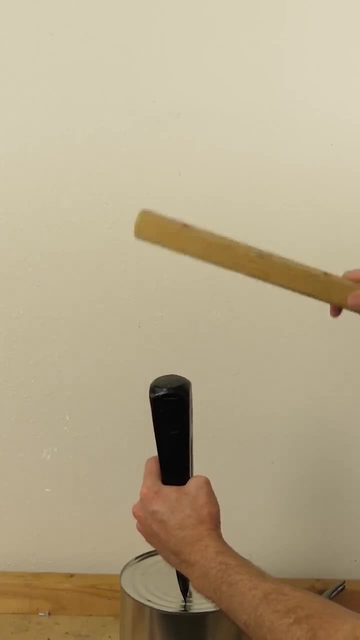 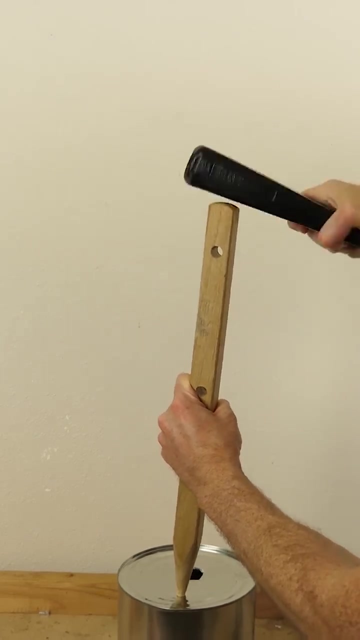 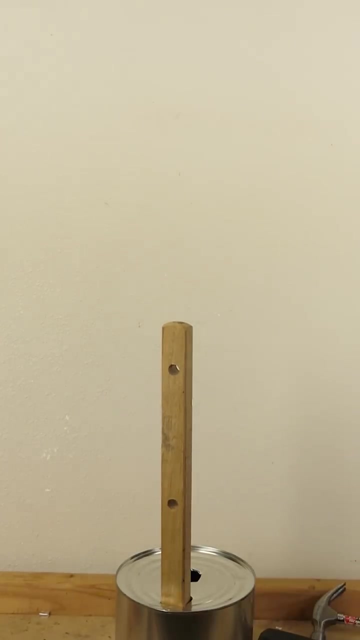 something with a larger mass. the momentum overall is small so you can't do much with it. But if I were to reverse the rolls and hit something with a large mass with a large velocity, then it easily transfers a lot of momentum to the smaller mass. So I definitely 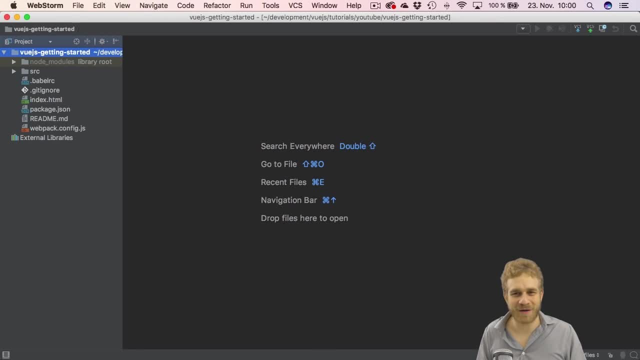 Welcome to another video on Vuejs 2.. Now, if you watched my last video- and you may be sure to fully understand this one here- you saw that I set up a local project using Vuejs with the Vue CLI, to have a workflow using Webpack to well be able to build bigger projects, to have a fully functional workflow which also allows me to split up my Vue code over multiple files.